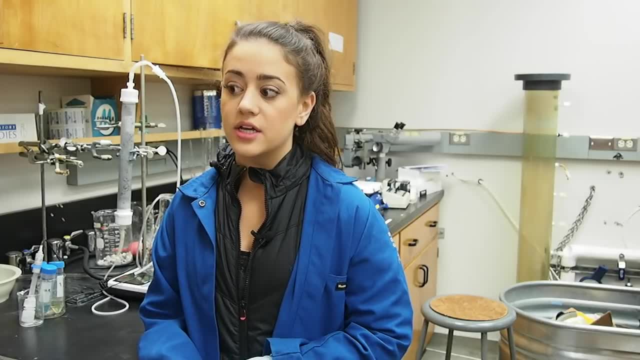 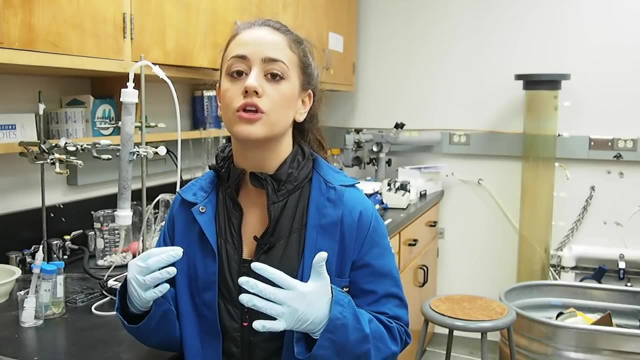 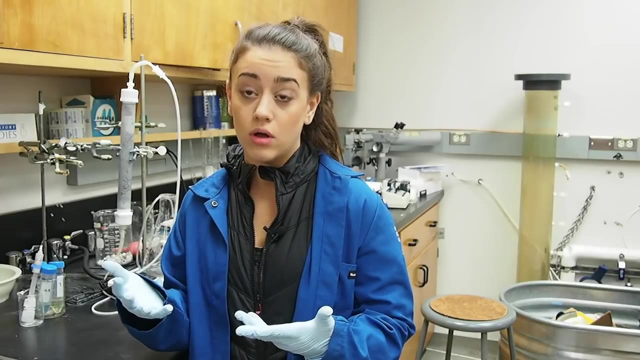 the box and be independent and find out information for yourself. If you have a question, you have to. you look online, you read papers, you become independent, The expert on something even as small as some new technique or machine, or you. people then are like: well, they ask you the questions and you're supposed to. 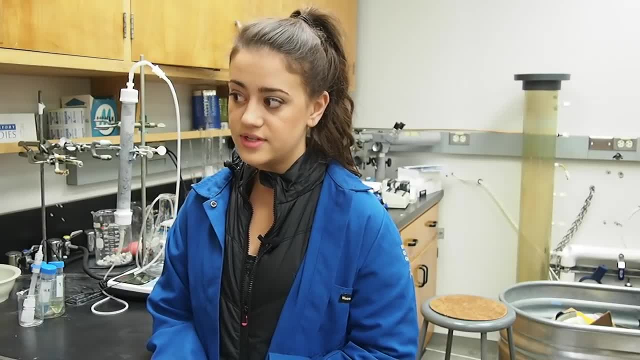 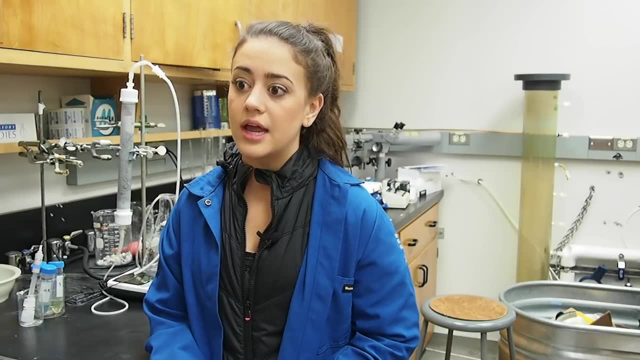 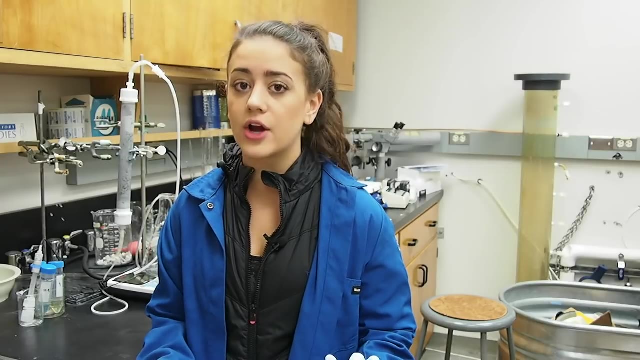 know, In undergrad I studied environmental science, with an emphasis in microbiology, and then I worked- though I was an intern- in a civil and environmental engineering lab and I honestly liked environmental engineering because it combines all the different sciences. Like anyone from any background to any field, 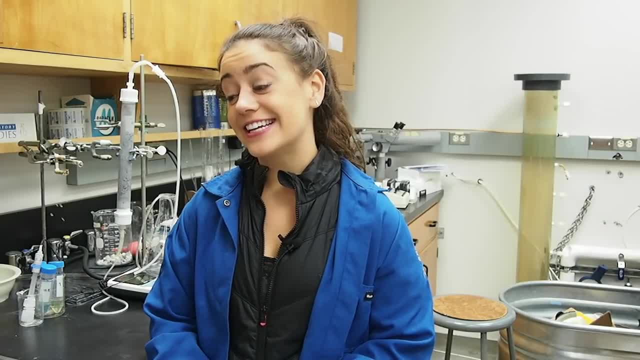 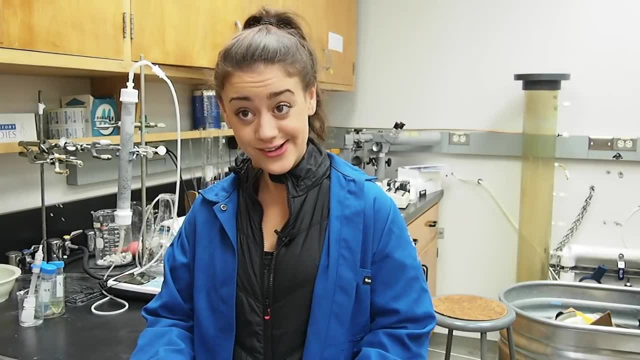 My mom is an environmental engineer and she works. she's a consultant and works. she pretty much implements the things that I research, which is kind of cool. That's awesome, Yeah, but that also means that she can call me on my bullshit all the time. 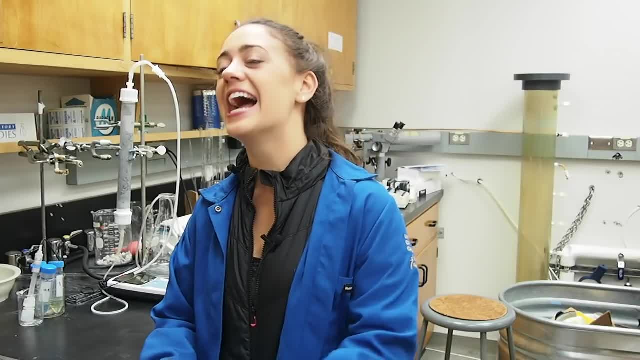 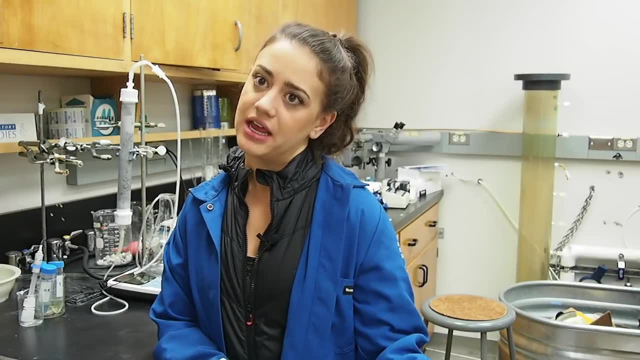 Like, oh honey, no, She's going great. Yeah, she was like no, it doesn't work like that. But I kind of resisted for a while. I was like mom, that's your thing. Okay, I don't know if I want to be anything environmental. 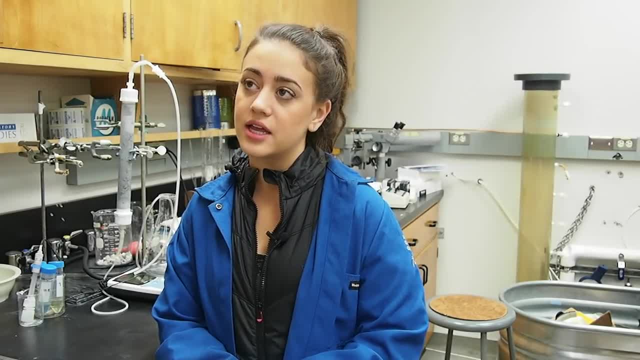 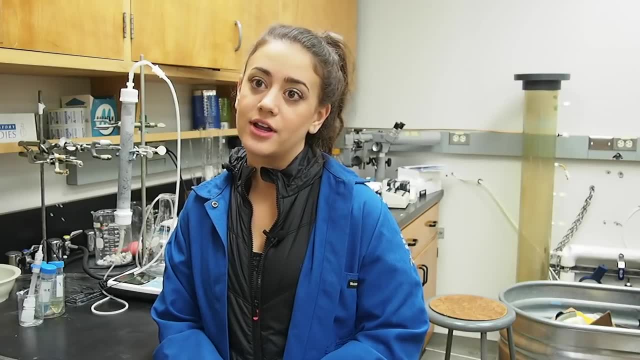 But it was meant to be, I think when she had me, like right after birth, like that afternoon, she was on like the phone with EPA talking. She's like, yeah, I just had a kid, But anyway, how's it going? How's the proposal? So like from the womb I was. 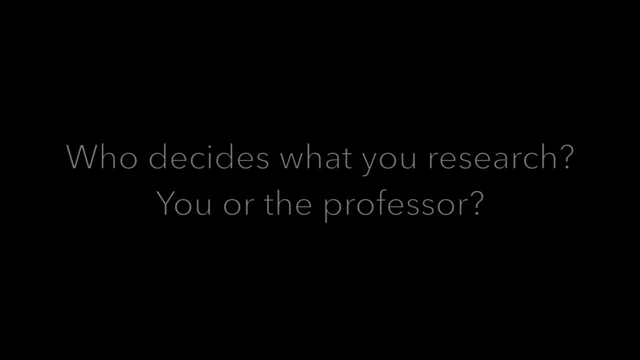 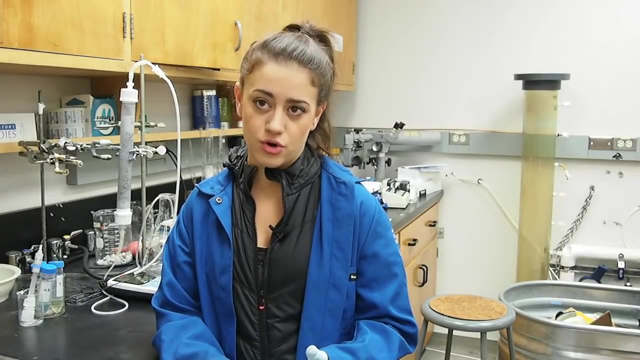 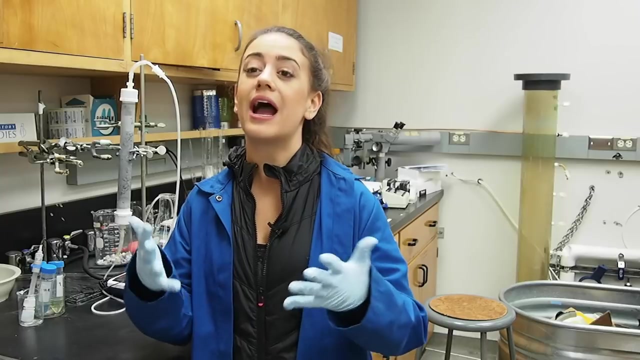 hearing about these things- A little bit of both. So usually when you come on to a team or in a lab, the professor will have some idea of what you're gonna work on. right, They have to fund you and usually the funding comes from a project and they'll be like: okay, here's, you have a. 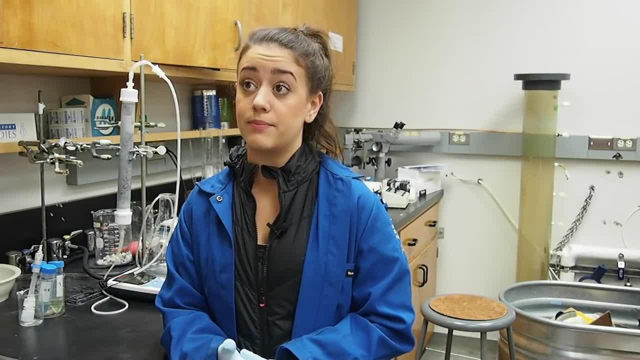 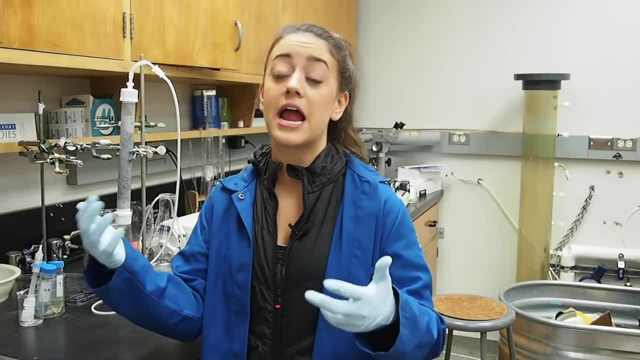 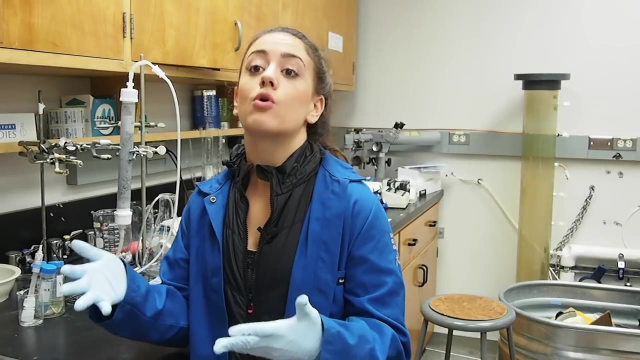 background that actually fits pretty well with this project. So, for example, I'm working on this project that's trying to like optimize bacteria for these harmful pollutants, And I had a background in that in undergrad and high school. And so my advisor is like: okay, here's a couple of 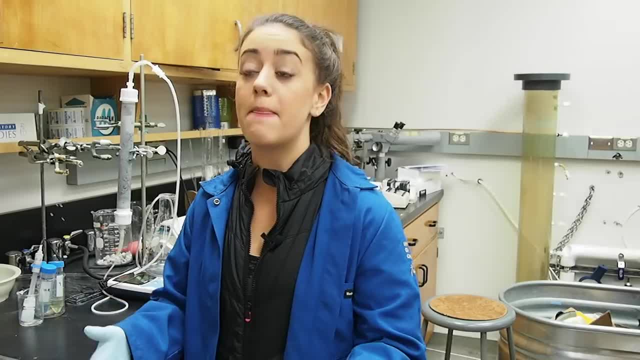 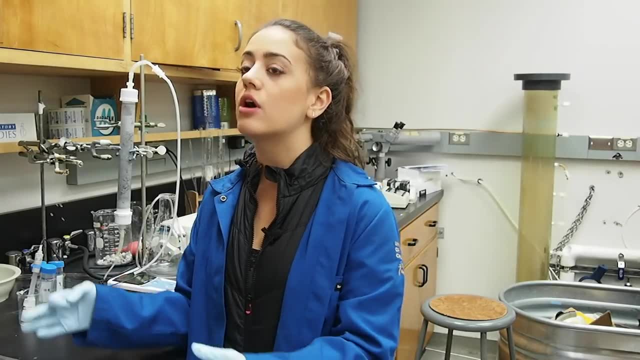 questions. Here's an idea we have. Can you implement this? And that's where then I'm the one, though in the lab, making the solutions, running the actual experiment, pressing the buttons, doing all the manual labor to get the answers, And then the professor is there to ask. 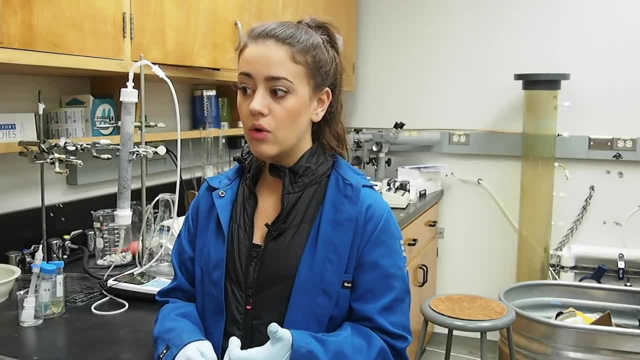 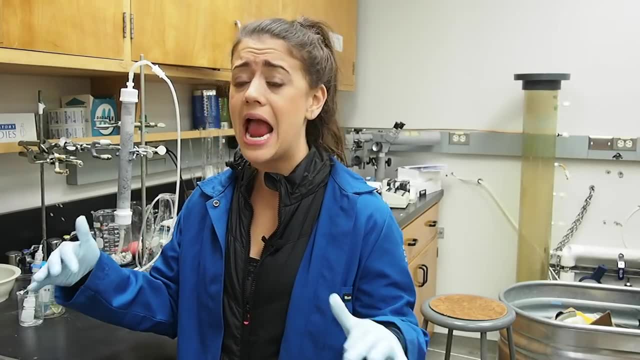 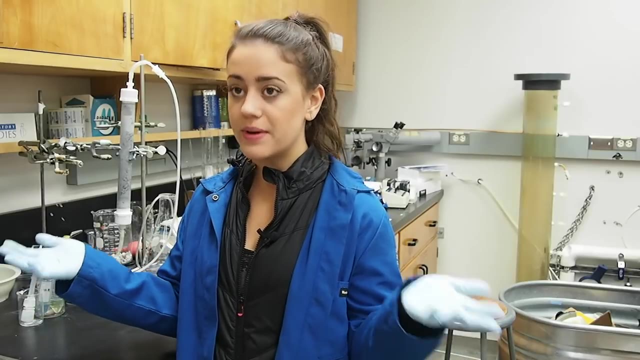 the questions of why, how and what's going on. So in research it's really you could spend all your days answering a billion type of questions That would be interesting to know, but unfortunately we're not paid to answer all questions We're paid to answer sometimes. 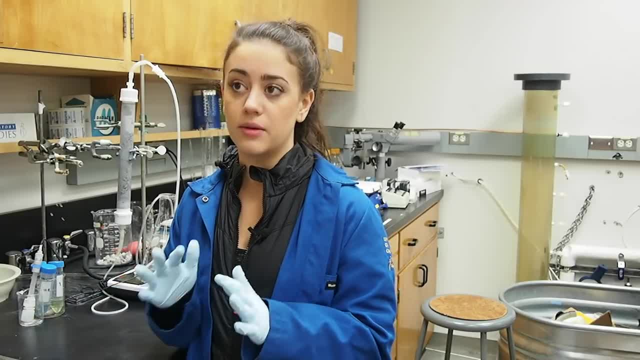 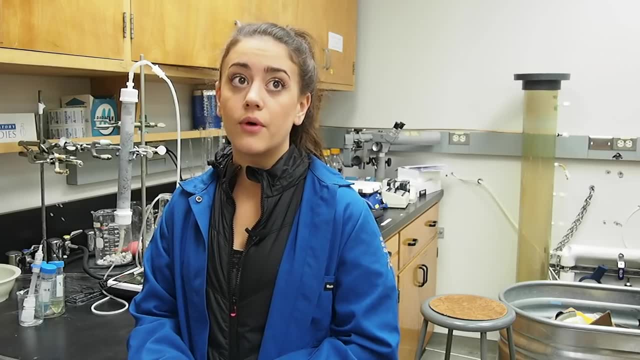 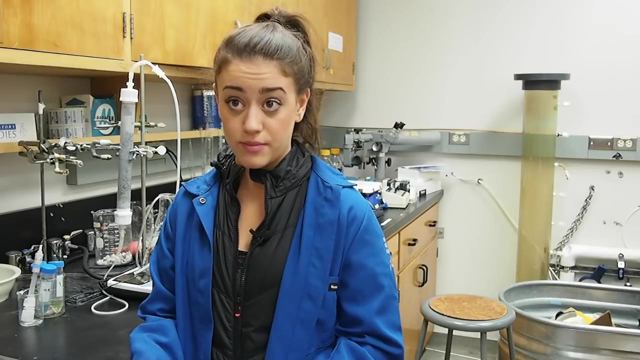 very specific questions And so you can get. that's the only problem. You can get in a little bit trouble if you start straying away too much. Yeah, So, for example, we work with like the med school, So a lot of times the things that they make actually can be applied to the environment. 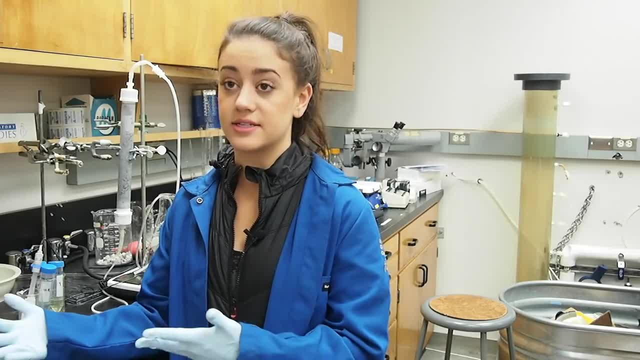 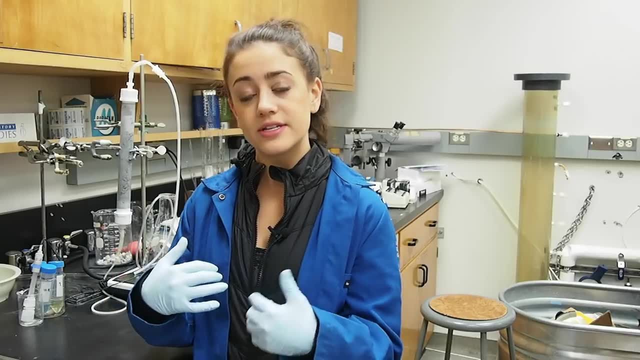 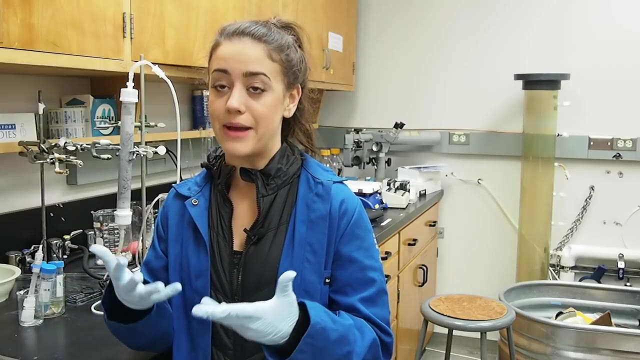 and to contaminants as well as maybe things in the body, And we work, which is kind of cool, And so we sometimes reformulate their ideas for our research. We also work with the biochemistry people and sometimes we'll help them understand bacteria. 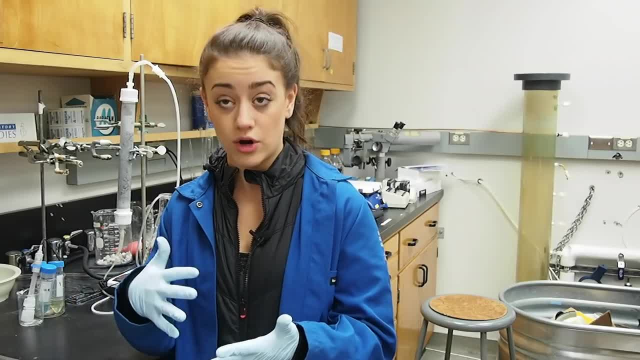 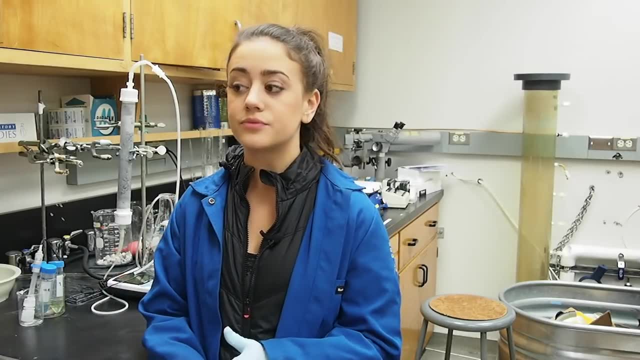 Like, for example, one of the people wants to try to figure out how to like filter water or like salt water, And they're trying to figure out how do I make it so bacteria don't attach to the filter And so they come to us and we help them. But remember, you always have to remember in this. 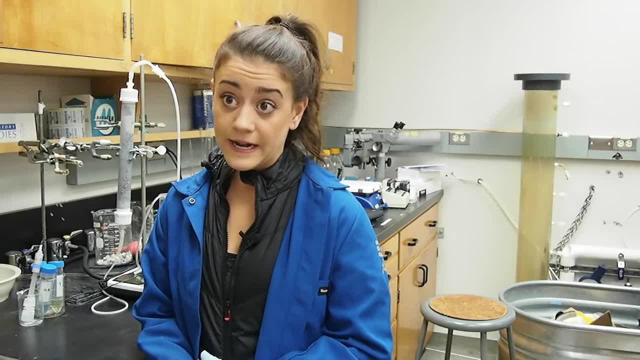 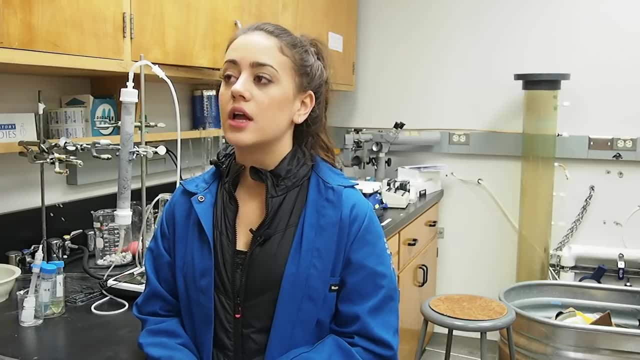 field, only one person gets to be the first author, really, And our line is about publishing papers and getting information out there, And so, yes, we definitely foster that, But at the end of the day, we still someone has to be the lead and 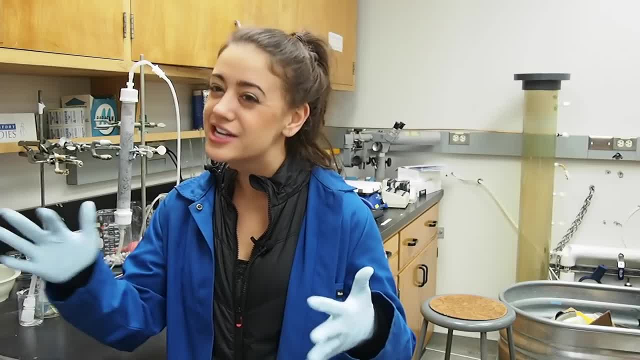 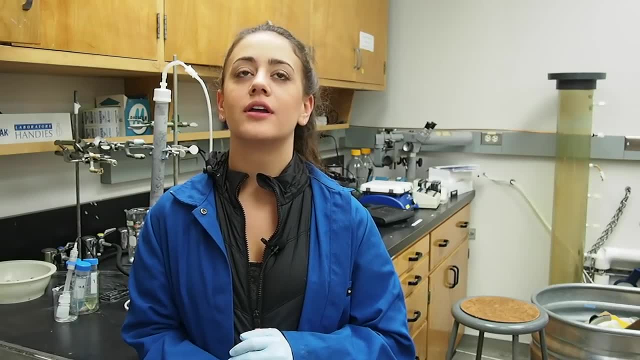 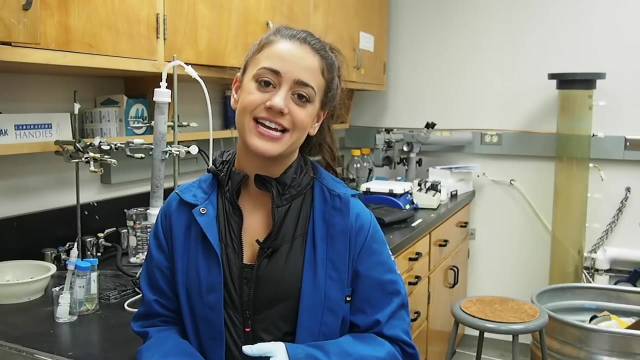 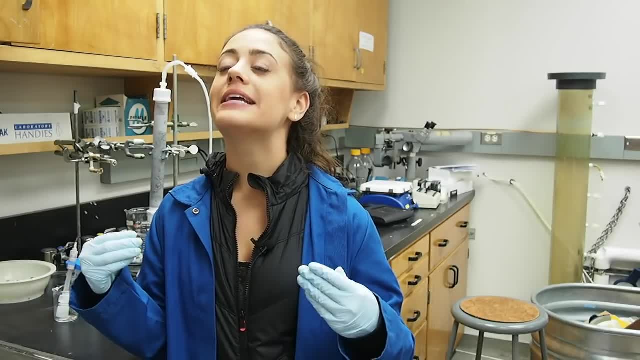 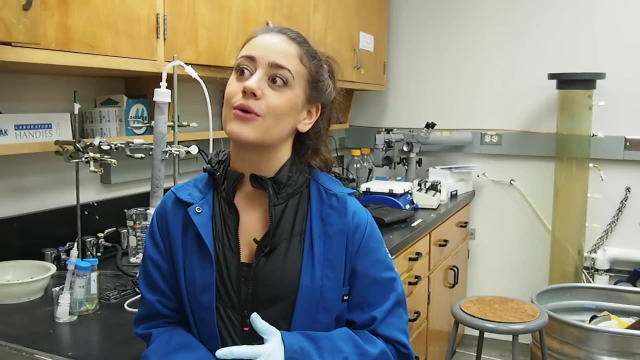 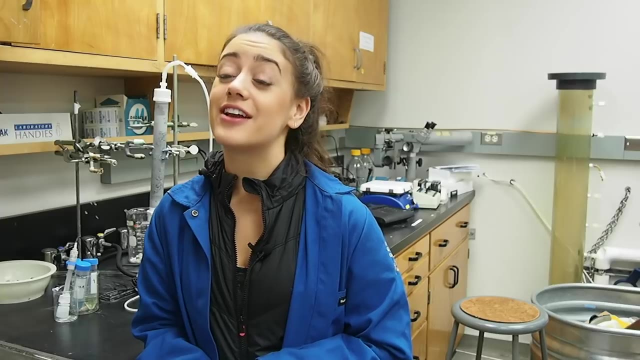 No one else knows yet And we're talking about all the really specifics that, honestly, no one else will probably ever know or want to know. And I feel like sometimes I'm in this own little world of science and of knowledge and it feels cool Like I know my family I have no idea, Like my brother has. 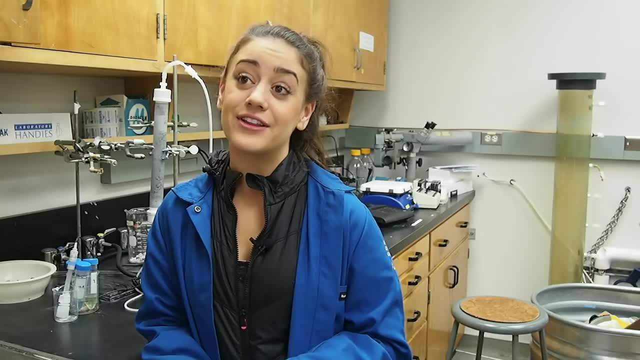 no idea what I'm doing and no idea what I'm talking about, but I feel like I get to enter this special little world and then I get to translate it to the public. No one else knows yet And we're talking about all the really specifics that, honestly, no one else will. 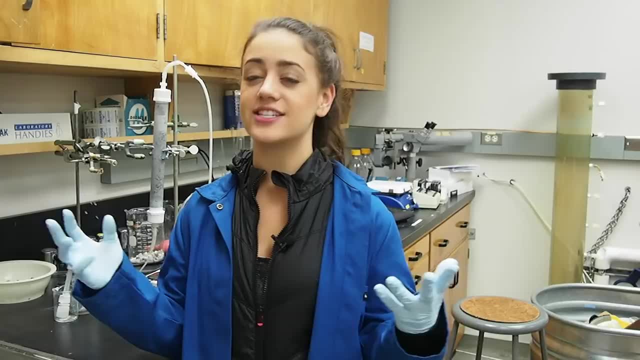 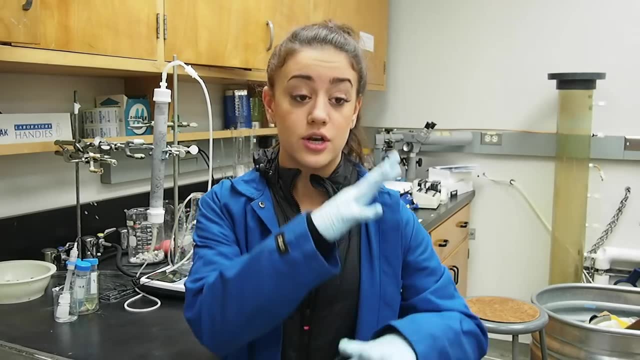 So it's like I get to be this bridge between the super specifics of why and how and literally every little detail about something, and then literally just put that into like a little package and present and then be like here. this is basically the idea. 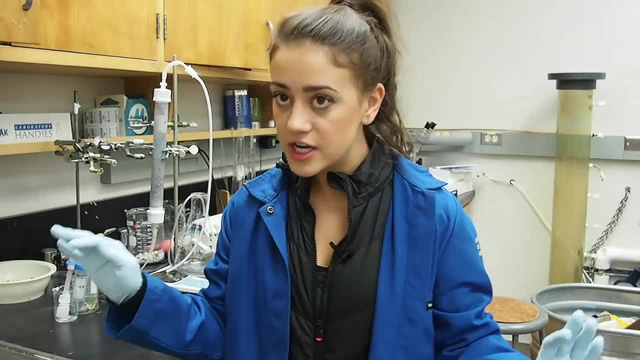 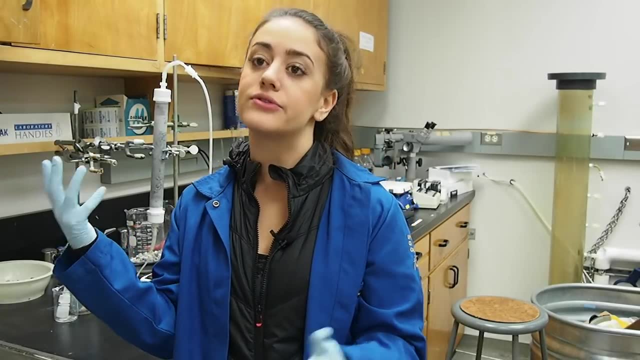 So it's like very few things you get to see from like start to finish, especially like maybe a corporate job where you're like your one little piece and maybe down the road you'll see something finished. But this is no, no, no, you don't get your degree unless you see something start to finish. 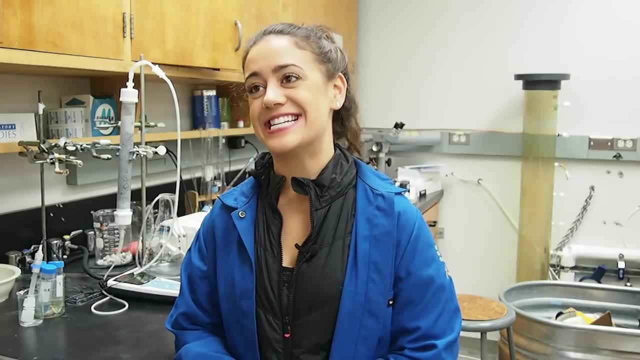 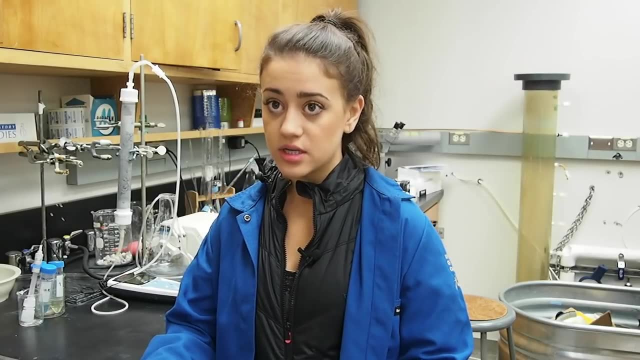 My personality, I guess, is very outgoing and I like being social, But also I like to kind of take myself seriously and my work seriously and I like to be the one to know why. I think if you're the kind of personality that likes to know why, 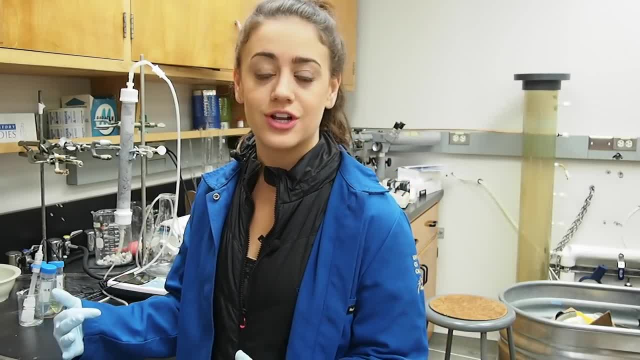 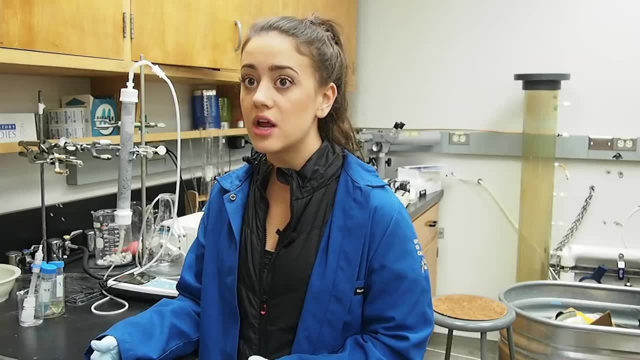 and you see something and you kind of do your own research, then I think exactly your curious mind. If you're kind of a curious person, I think this type of work you'll really enjoy and you have to enjoy it to do this work. 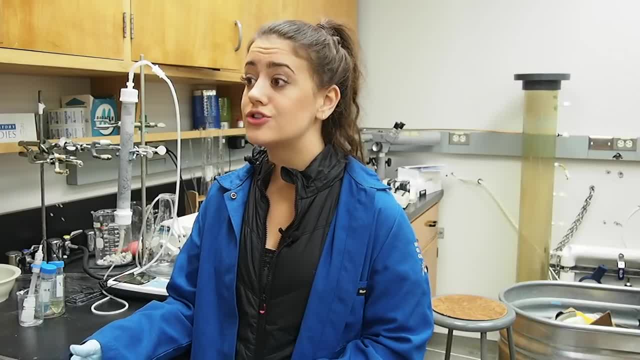 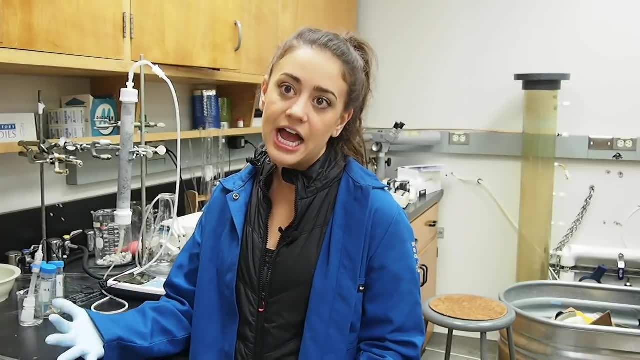 because six years is too long to just do something like, yeah, I'll get through it. right, You can get through a job, or maybe for a year, a year and a half or okay, But for this type of job you really have to love what you do. 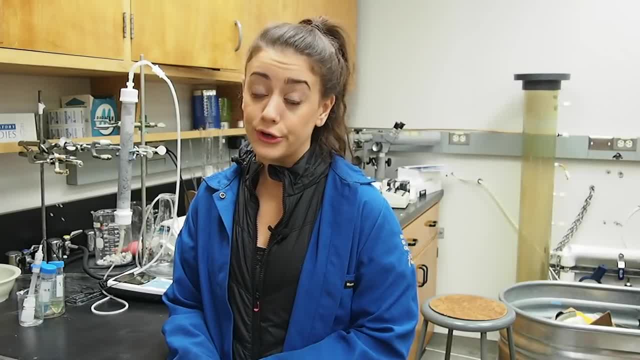 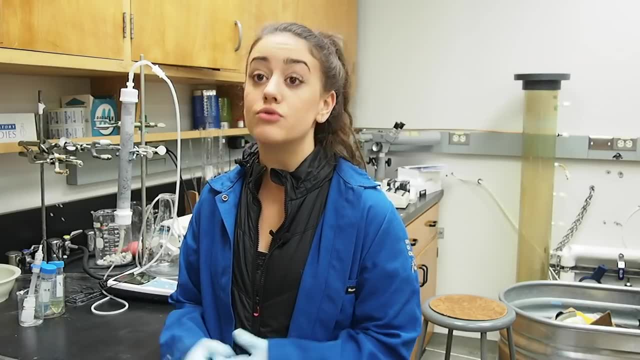 because we don't get paid a whole lot and it is a very long time and sometimes frustrating. We don't get, sometimes we don't get answers and you don't know, right, All the questions I'm answering no one knows And that's kind of unsettling, too right. 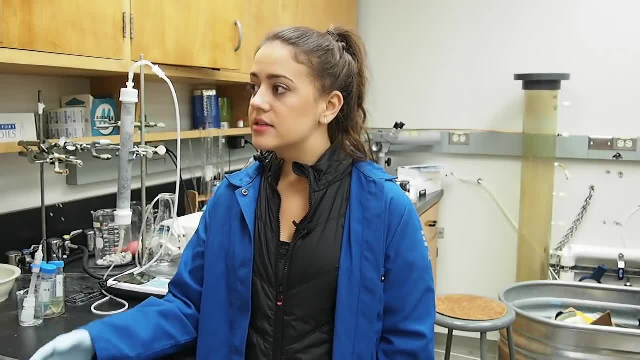 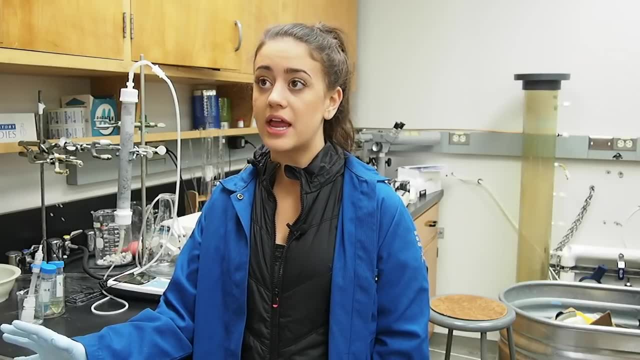 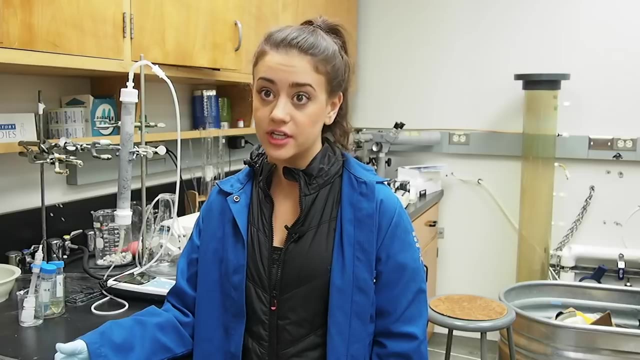 You're like: oh, I'm used to having some type of answer, someone to tell me the answer, And so a personality that is okay with that is okay with chaos is okay with. I've learned also that you have to have really good time management skills. 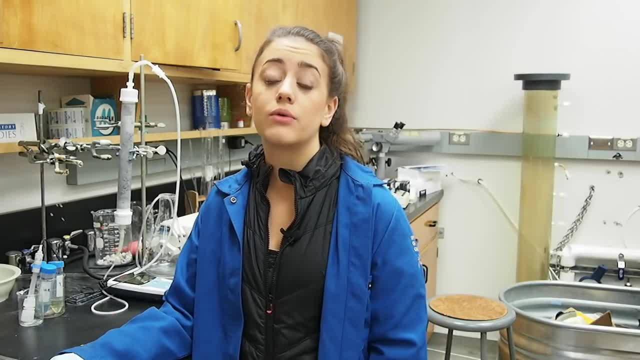 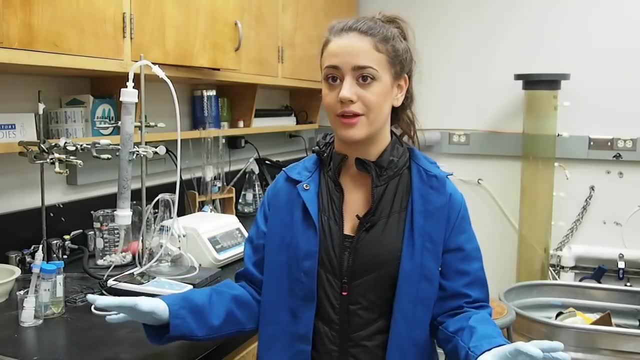 and a personality that is okay with that. You have to have a personality that is organized, but you get to a point where you have so many things on your plate that you can just handle stress and anxiety and just kind of like step back from it. 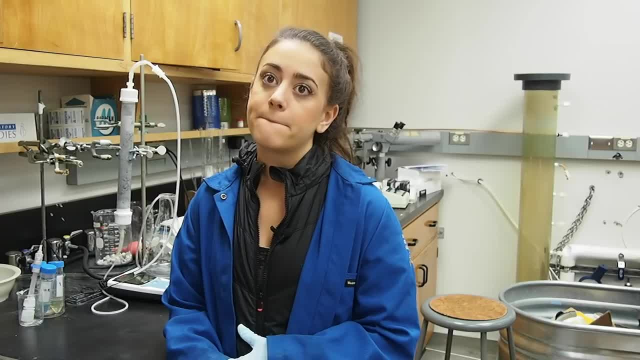 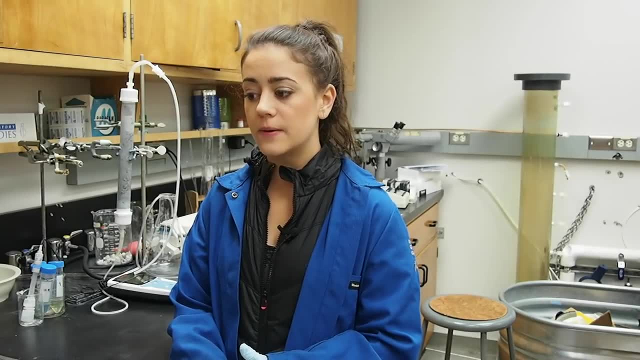 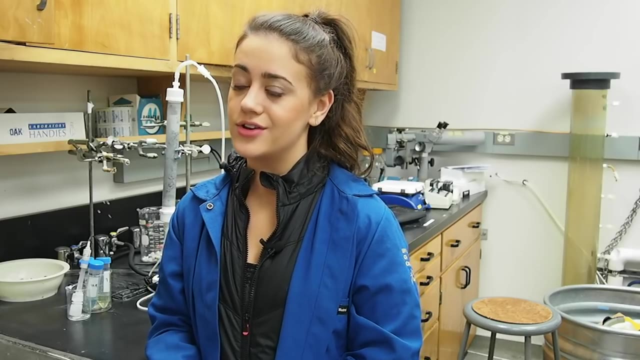 Confidence too. it's really good to have confidence, Otherwise no one here is going to give it to you, And so it's kind of a harsh reality. I had to learn, but a good one, a good one. I won this recent award called the New England Biolabs. 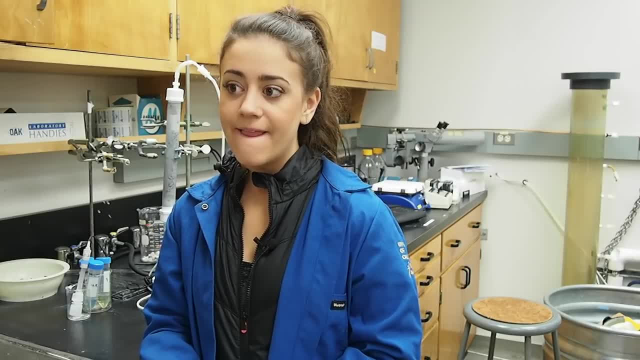 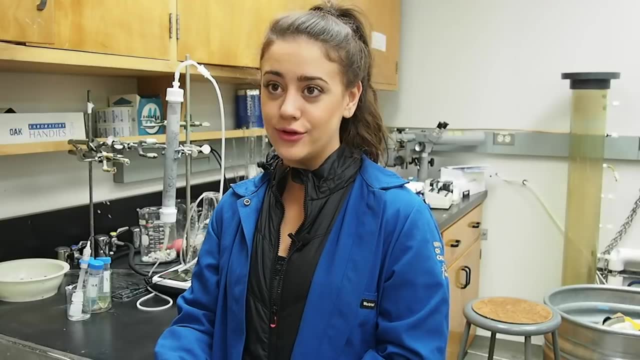 It's a passion and science award You had to give like a little TED talk. It felt it was like the first presentation where I felt like someone wanted to hear from me other than my lab group or other. everything else I've ever done has been: 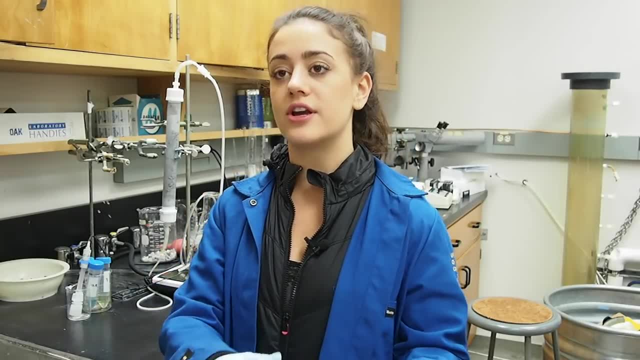 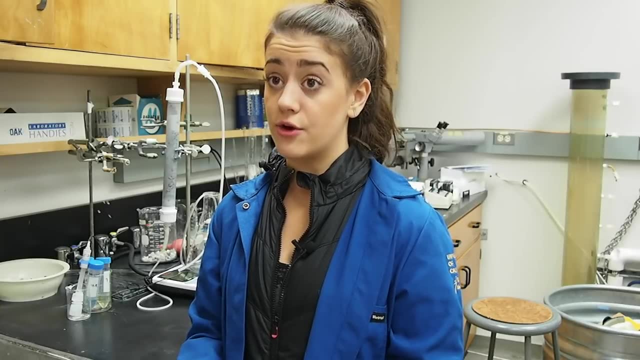 okay, you're applying for a grant. here's writing: great, you got the money. oh, sorry, you didn't get it. This is the first thing that was like: we're going to value you because of your passion, your dedication, and we want to hear from you. 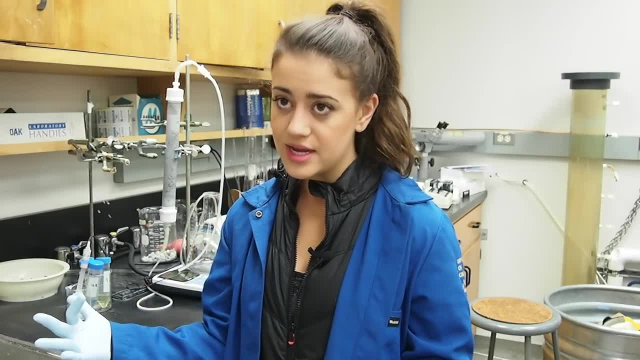 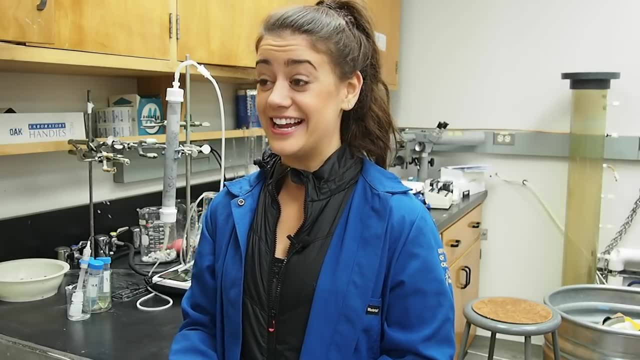 And they give you like a travel, a little travel grant. but this award was not really about the money. It was more about like we want to get you out there as a communicator, as a scientist, And I got to talk to this like huge audience and it felt it was like the first time where I was like 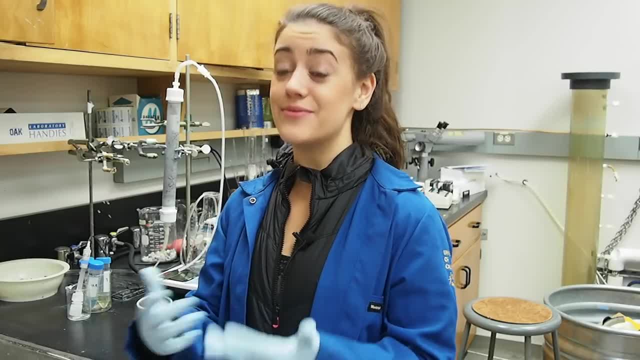 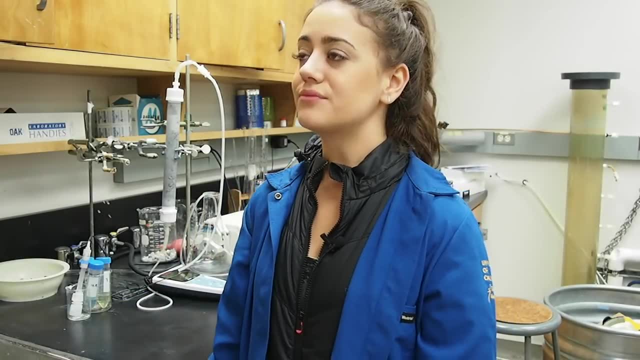 wow, this is what it feels. this is what it's supposed to be like of communicating just to everyone and of any background, and not just like at a conference. right, We have like a very select group of people that are trying to criticize your work. 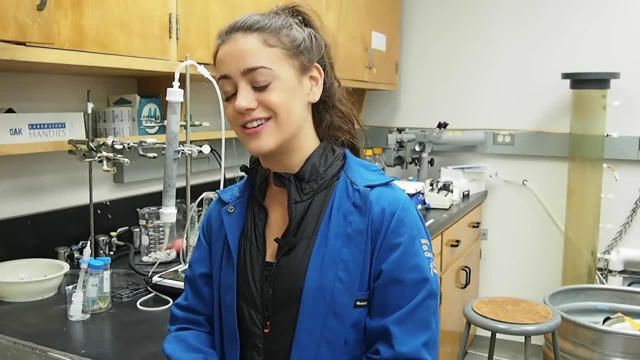 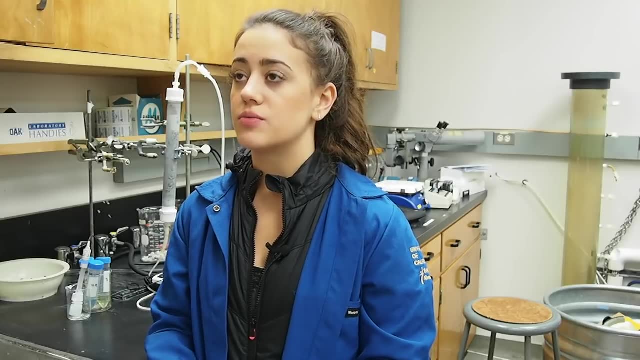 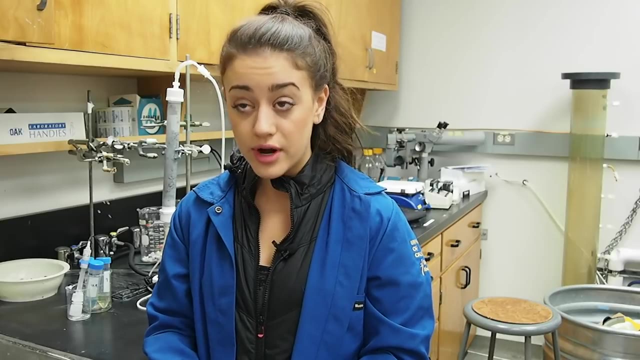 These people were like: wow, what are you doing? This is cool, That's awesome. I think It's. being a woman in science is becoming much more prevalent and much more accepted and much more desired, which I think is really great. 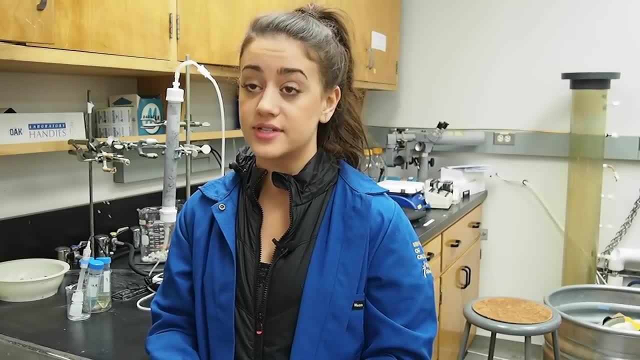 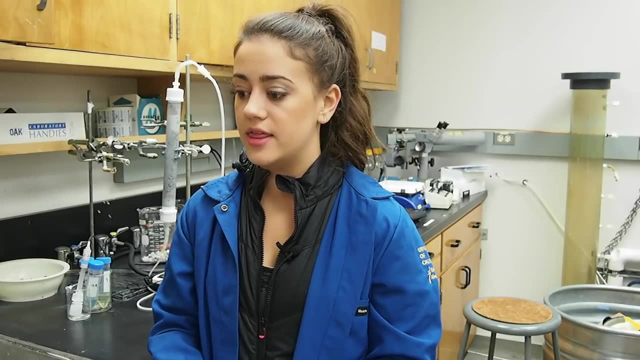 I think it's really cool. There's a lot of women's scholarships, There's a lot of emphasis on having women in engineering and keeping women in engineering, and that's a really good thing, I guess, if you're thinking about this career. 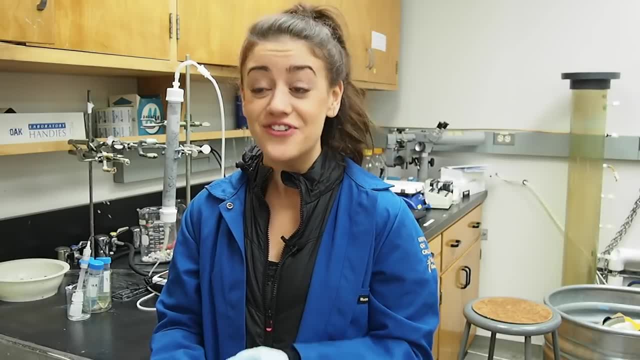 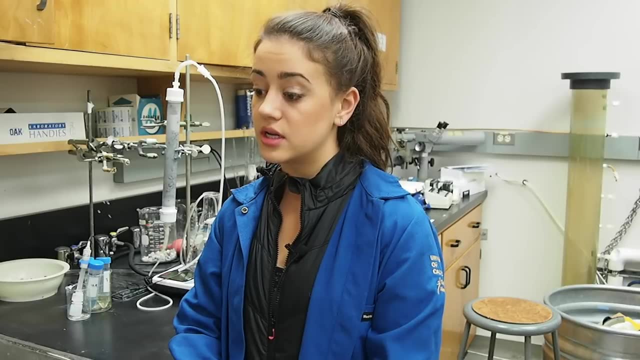 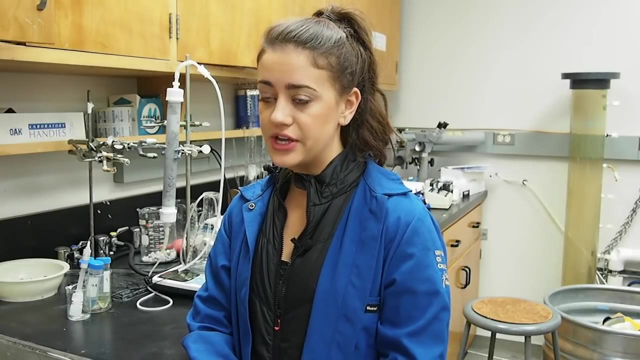 is that you were wanted and you're desired and you can do it. I would say, my biggest mentor besides my mom was in high school. I worked in a lab that had a high school internship thing And I remember the PhD student was a woman and she took me seriously. 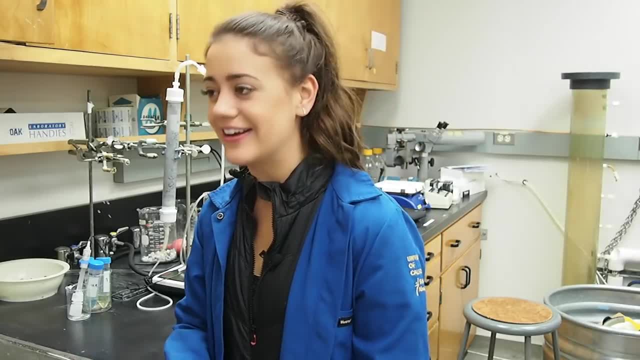 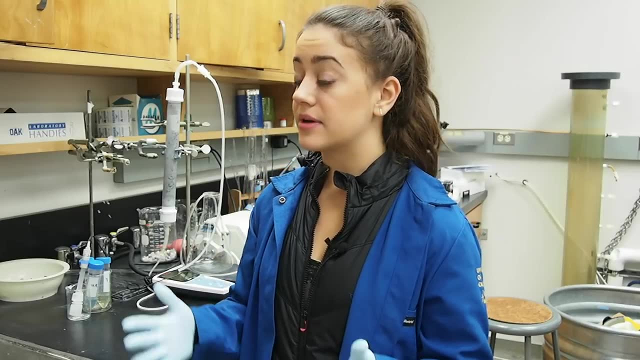 And as a high school student we kind of joke. We're like, yeah, they can't do anything. I can't trust high school to do anything. But this person for some reason took me seriously, was like I'm going to teach you these things. 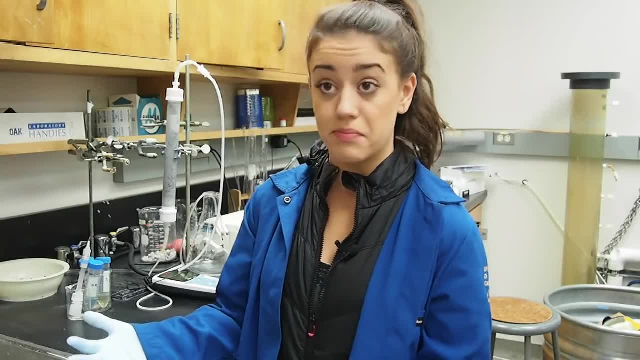 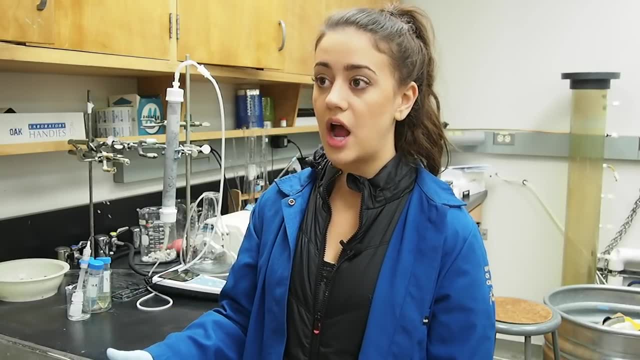 I had no idea whether or not I was going to do something, whether she was teaching me things that were advanced or basic. I was like this is great, And I think that started my curiosity. It started me. I was like, oh, she takes me seriously. 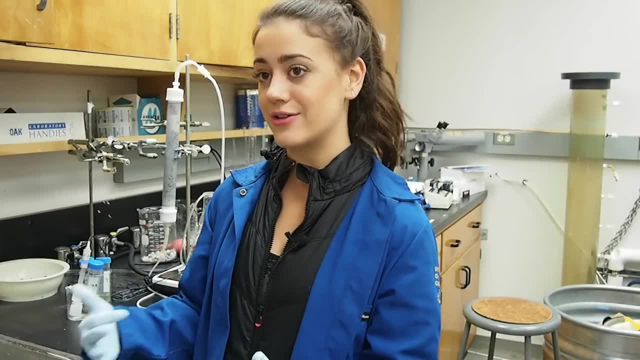 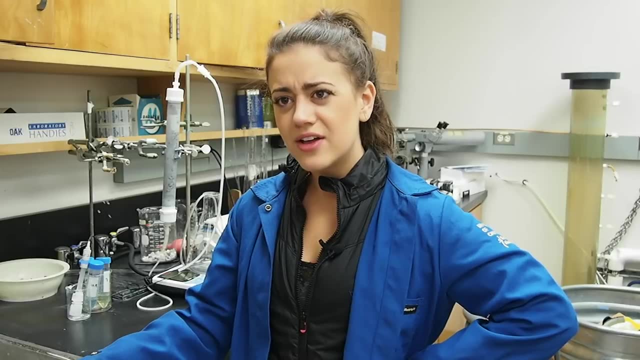 I should take this seriously And I'm curious. I wanna do my own outside research. And then in college I had a female mentor as well. I had a lot of female mentors And my advisor now is female. It was cool to see if a strong fan in science I guess. 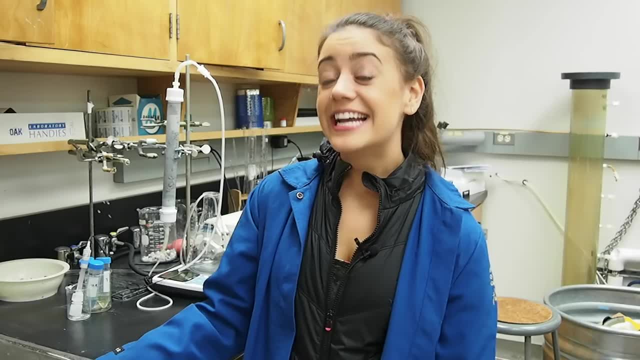 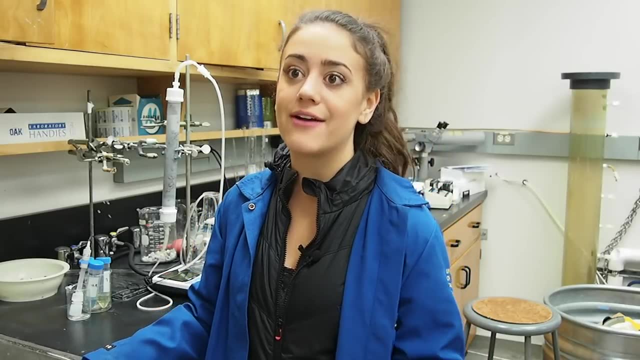 Like literally, they've all been super supportive of me. Yeah, so I TA an introductory environmental engineering course and that's really cool because you get to advertise your research And hey, if anyone wants to work in the lab, come talk to me. 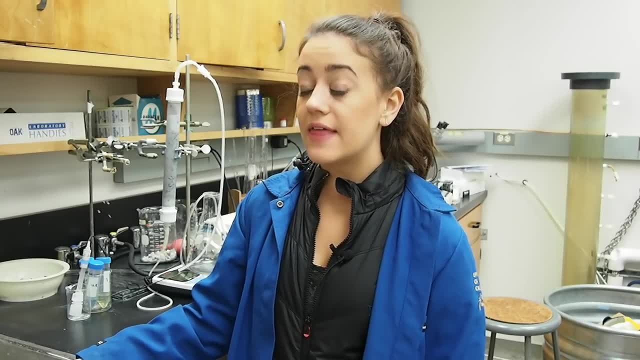 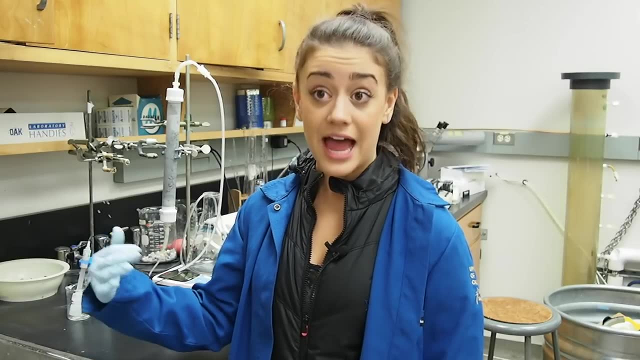 And I hold like a little seminar for my students And then I also mentor right now one girl. she's in environmental science and is applying to grad school right now And she's been in the lab and works with me for the past like eight months. 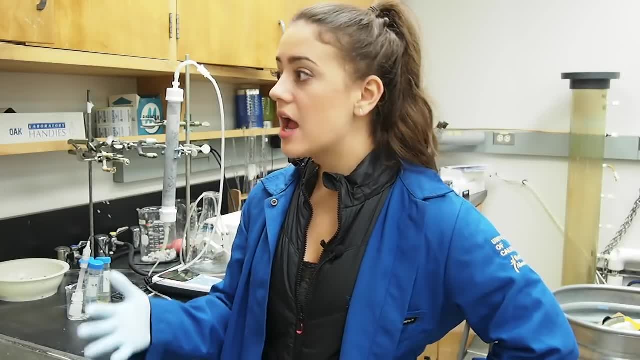 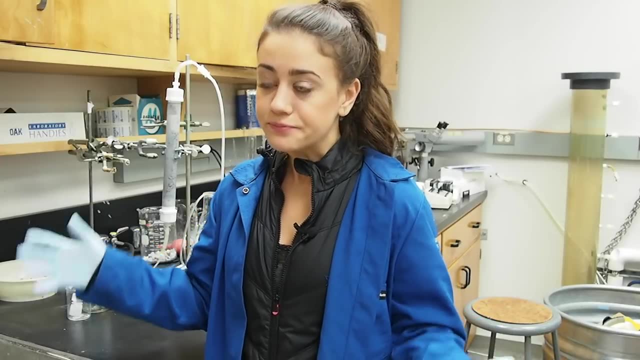 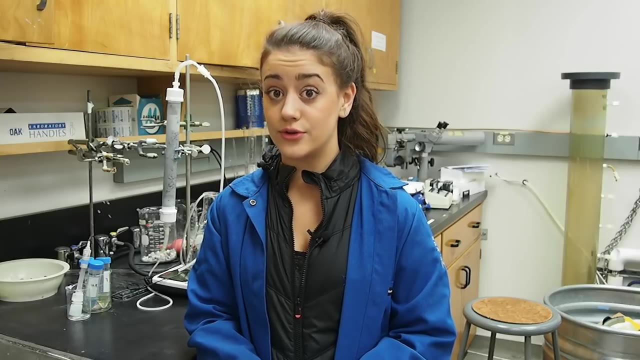 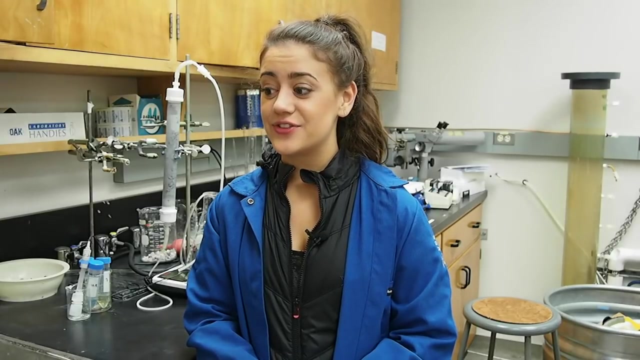 As a mentor, you teach them everything. Not only teach them how to make something, but also reasons why. Always explain reasons why, Otherwise you forget. I would say: don't overload yourself. I think it's really easy to do And don't freak out. 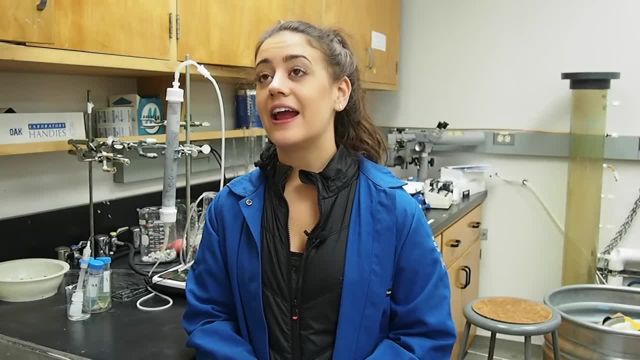 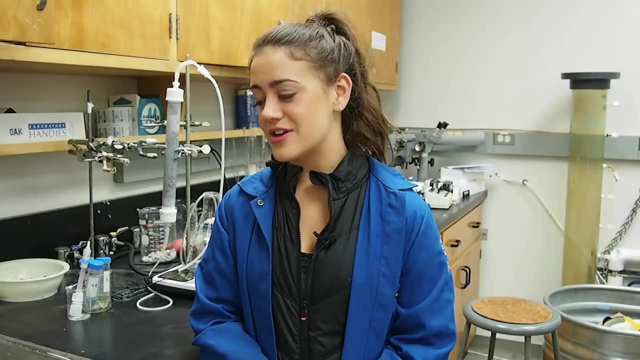 It's okay. I feel like I freaked out a lot Like oh no, And you look back you're like, oh yeah, that kind of passed and that was okay, So it's all going to be okay. 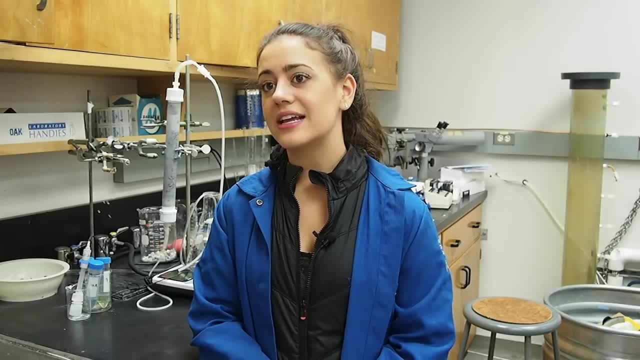 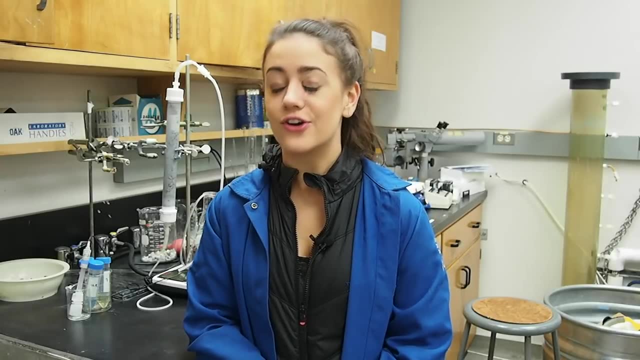 And it's okay to like get a no and it's okay to fail. I think failing is part of actually having great success. I've done a lot of it, So yeah, I don't know what to say. That was good. 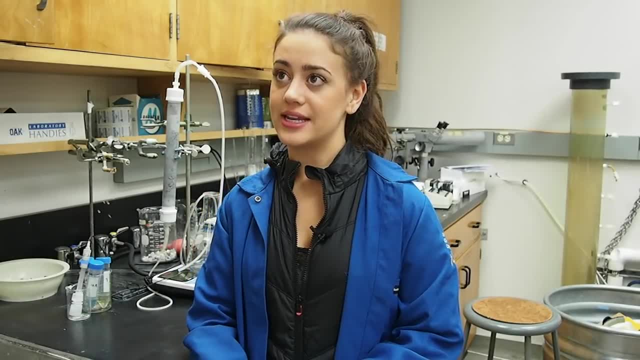 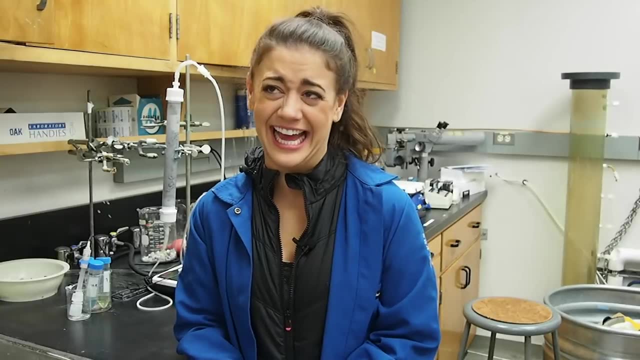 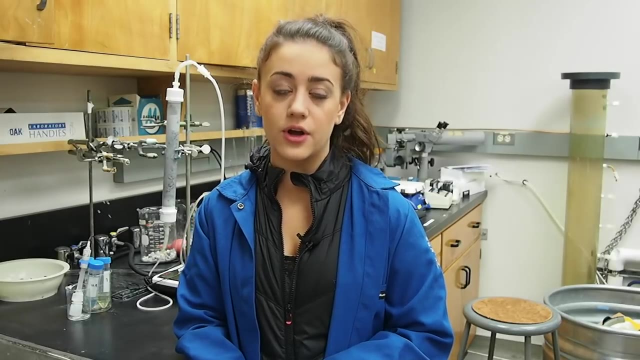 If you want to reach out to me, Alex Polasco, you can email me at apolasco, at guclaedu. Yeah, that You don't have to write that down. Do you have Twitter or Facebook? Have Facebook? Absolutely, reach out Facebook or Instagram.